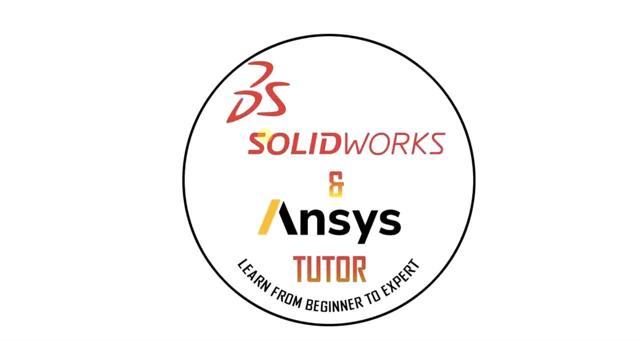 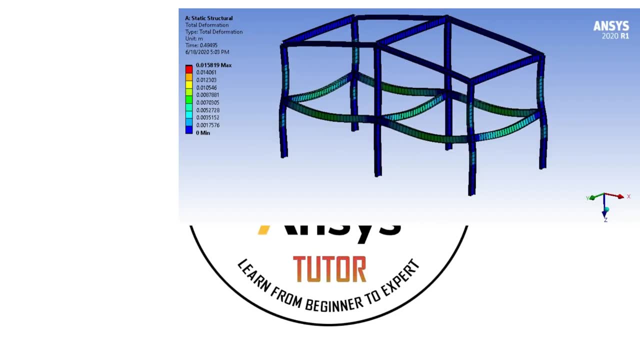 Hi guys, welcome back to ANSYS Workbench Tutorials. In this tutorial we are going to solve Frame Structure Analysis and we are going to make the geometry in ANSYS Space Claim using Beam Profile. So before starting the video, if you are new and haven't subscribed our channel, 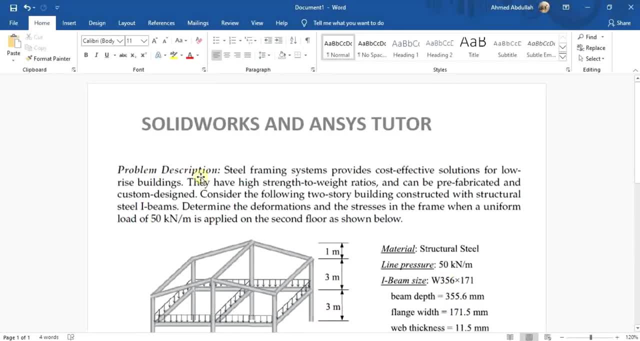 press the subscribe button. So this is our problem description. We are going to solve a two-story building constructed with structural steel I-beams and we will apply uniform load of 50 kN per meter and we will find the deformation and stresses. This is our geometry and this 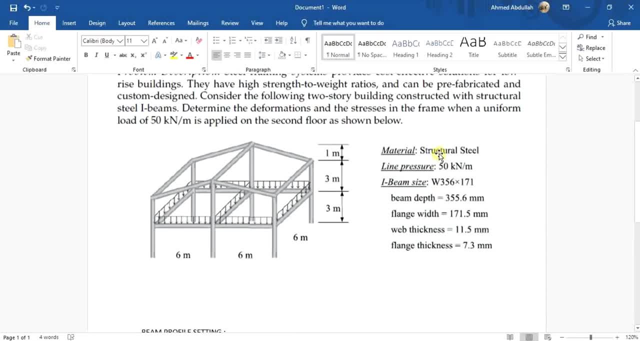 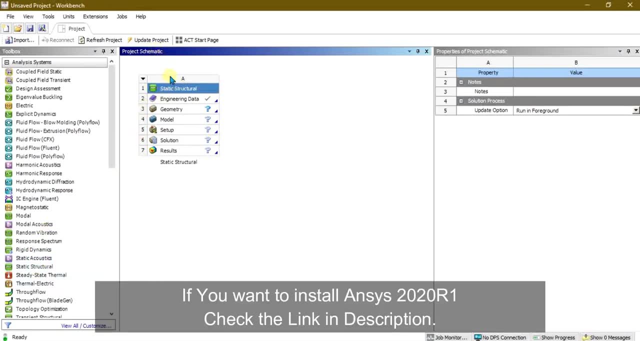 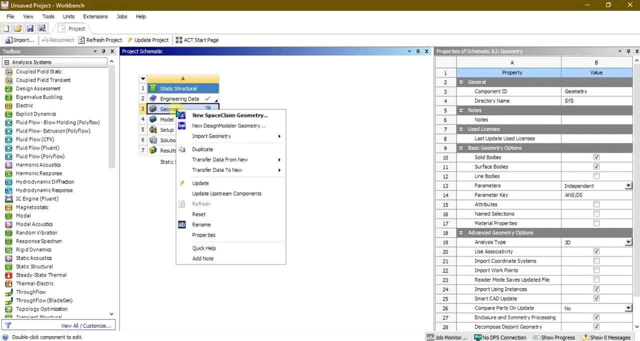 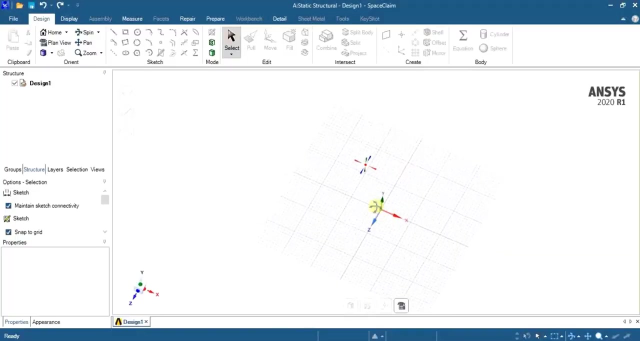 is the material we are going to use: structural steel. So let's start. First of all, drag static structural table in project schematic. Then right click on geometry So select new space claim geometry from here. So when your space claim have been opened, 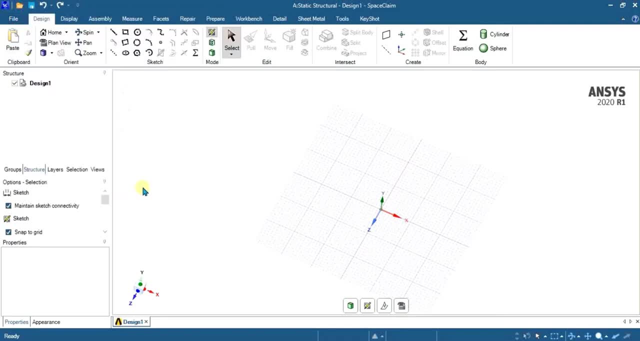 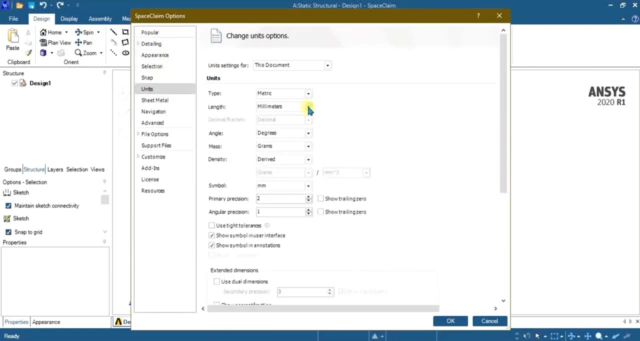 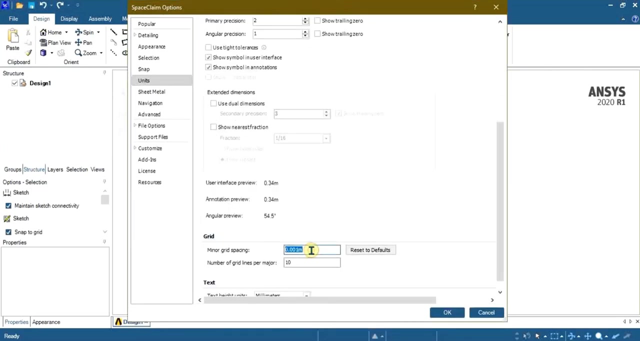 go to files, go to space claim options to set your SI units. Already it is in millimeter. We are going to select it in meters because our geometry is in meters and we will give the minor grid spacing of 1. And primary precision of 4.. So select ok from here. Now select plane view like this: 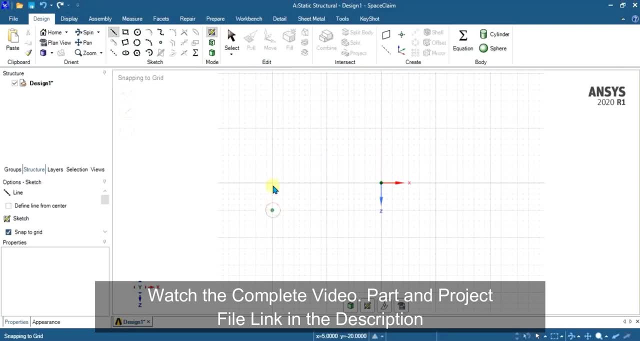 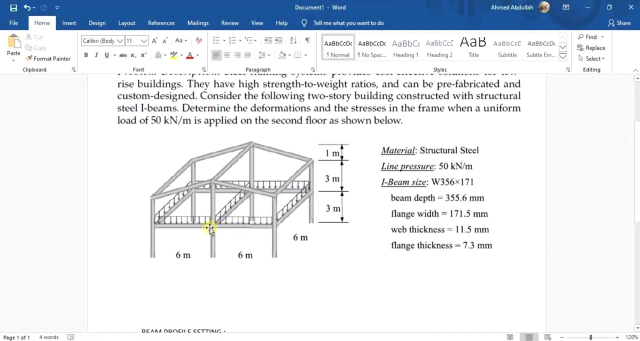 And select line from here And make the line of 3 meters. Let me show you. So our vertical length is 3 meter and our horizontal length is 6 meter. So, first of all, we are going to create a plane. So we are going to create a plane. 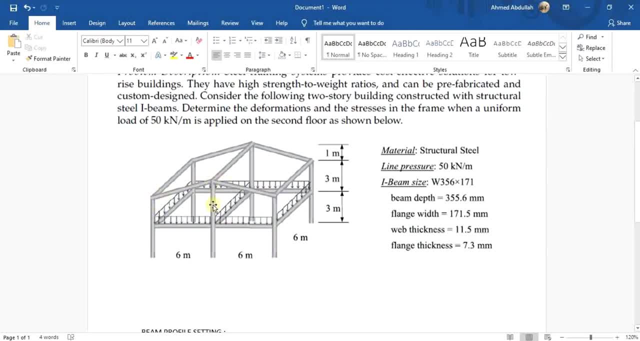 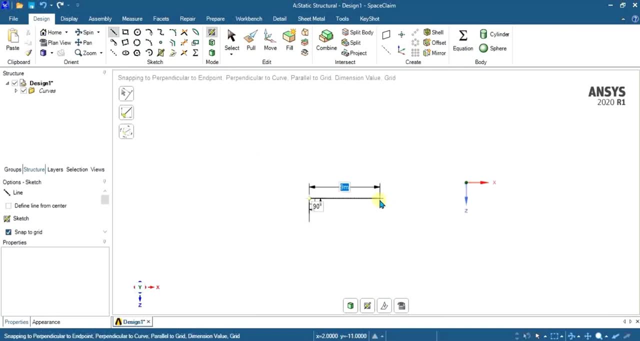 So first of all we are going to create a plane. So our vertical length is 3 meter and we are going to make this sketch and then we will mirror it and make the 3D. So now we will make the length of 6 meter like this. Follow the steps to make the geometry. 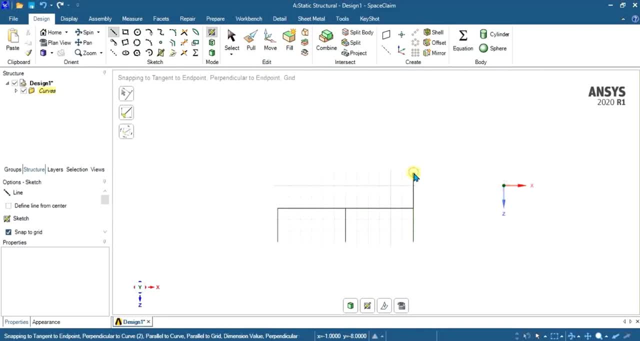 exactly. So, as you can see that our first part is ready and we have made the sketch, Now go to 3D mode, Select, move from here And create a plane, Select the surface. Now you can see that our plane have been made. 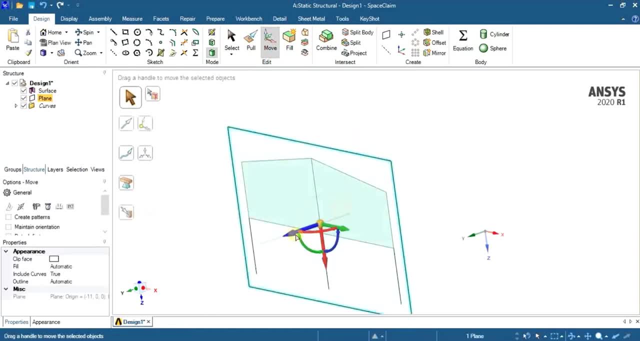 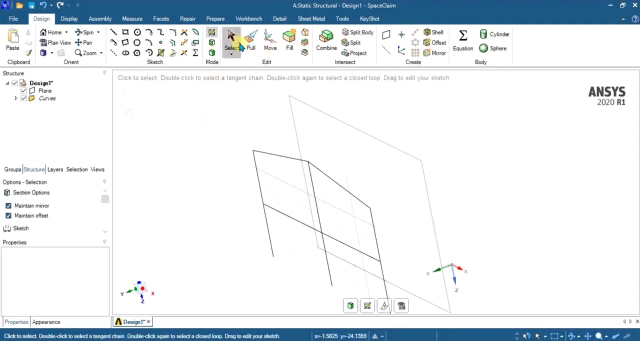 We will pull this plane and give it the value of 3 meter, like this, And we will mirror this sketch with reference to this plane. So go to edit sketch from here And select mirror. Select this from here And select the mirror body, Brag the rectangle And, after bragging the rectangle, select this: 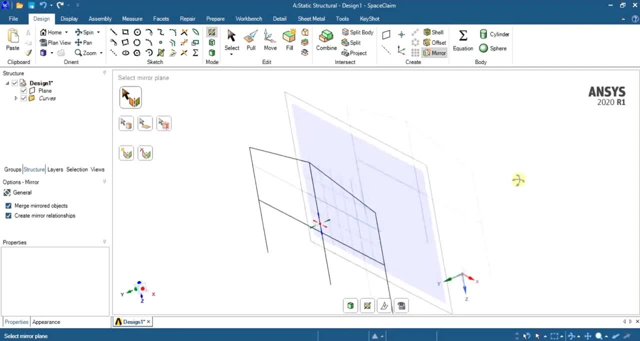 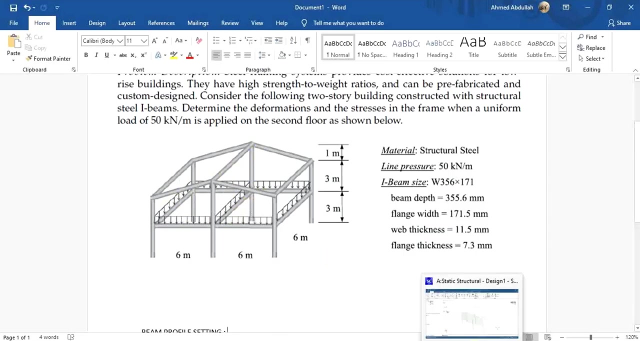 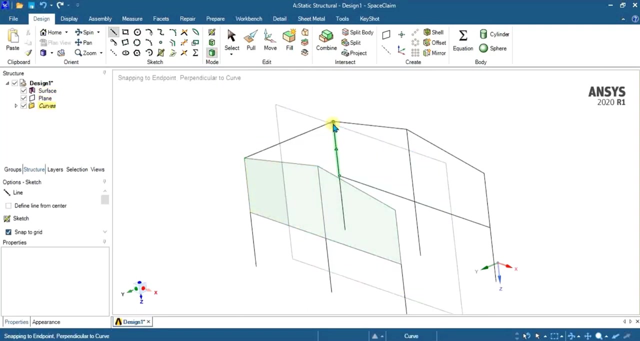 plane like this. Now you can see that our geometry has been created and mirror along this plane. Exit this. And now what we will do is we are going to make the internal lines to join these two sketches. For that we will go to 3D mode and select this point and this point. 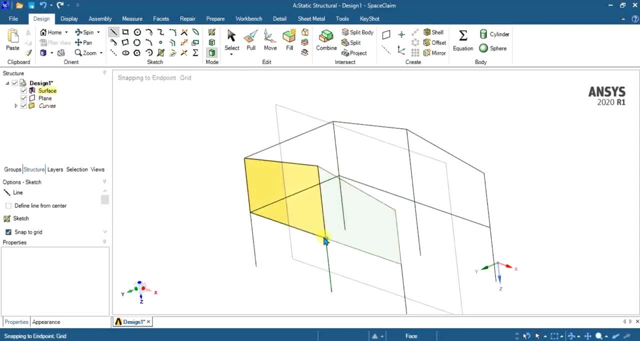 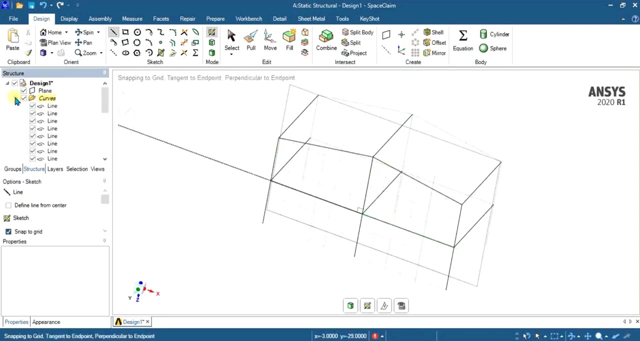 After that, select this point with this and make the lines accordingly And click 네 to confirm. So you can see that our structure is ready. So now we will apply beam tool For that again. go to edit sketch And go to lines. Select all the lines from here. 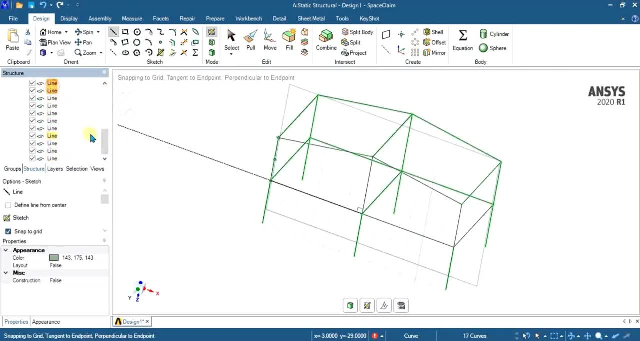 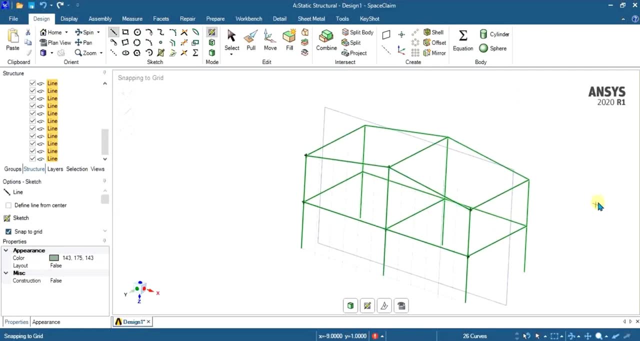 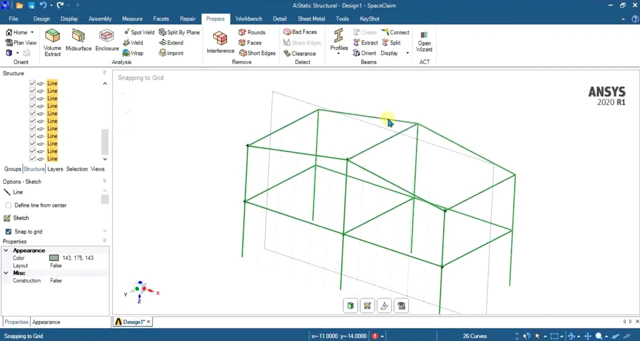 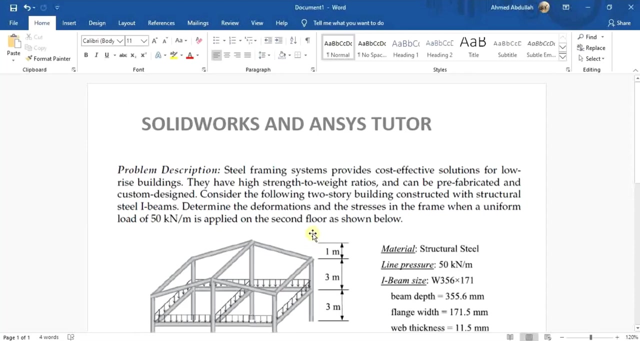 And make it 3D. so our all lines have been selected. now what we will do is we will go to prepare and select I-beam profile from here. so after selecting I-beam profile, go to beam profile and select edit beam profile to edit the dimension of this I-beam. so we are going to give these. 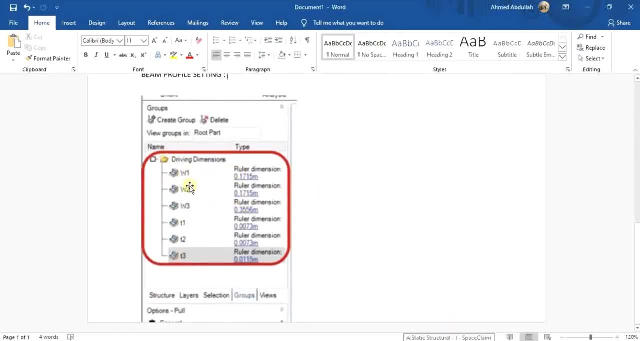 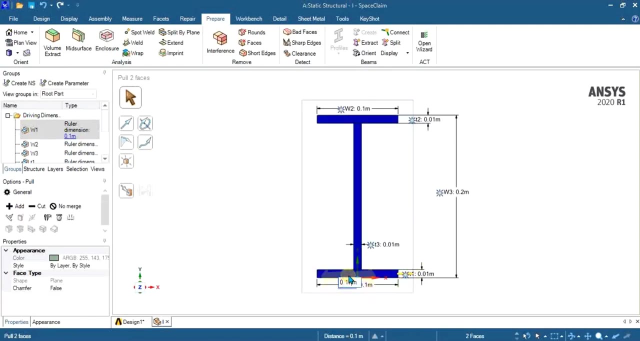 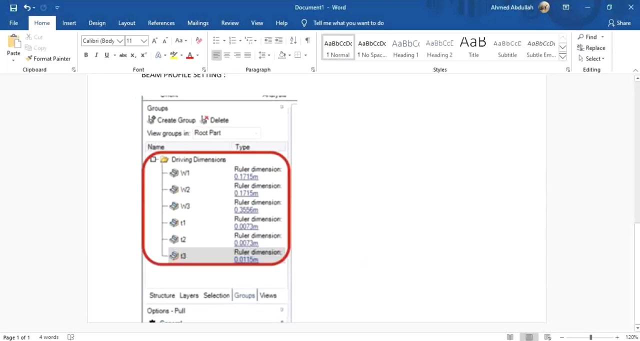 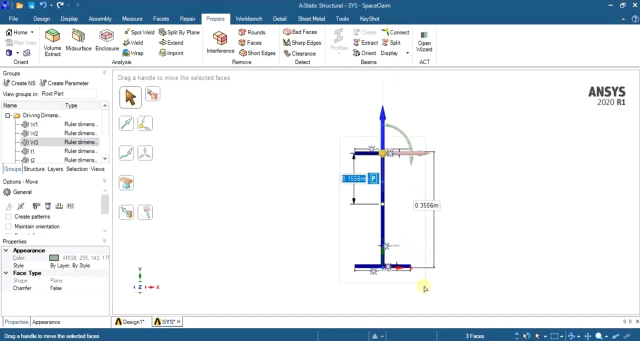 dimension to this I-beam. so our width one and width two of 0.1715 meter, as given in this problem. double click on width one and give here the value of 1715 meter. again repeat the step for all the values. Thank you.